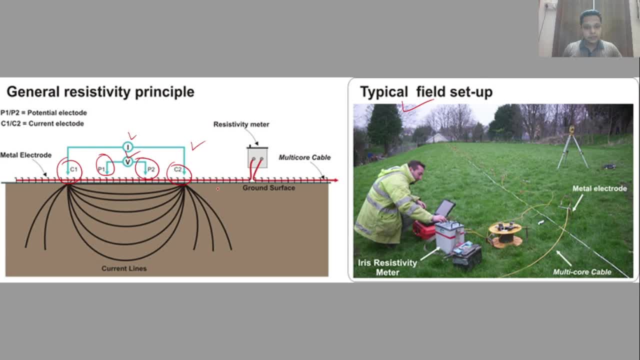 but multiple electrodes can be used and can be laid down. the keep by using cables for hundreds of kilometers, And an effective survey of 100 square kilometers can be done using this technique, And also the depth of penetration is quite good because you can get an idea about up to several kilometers. 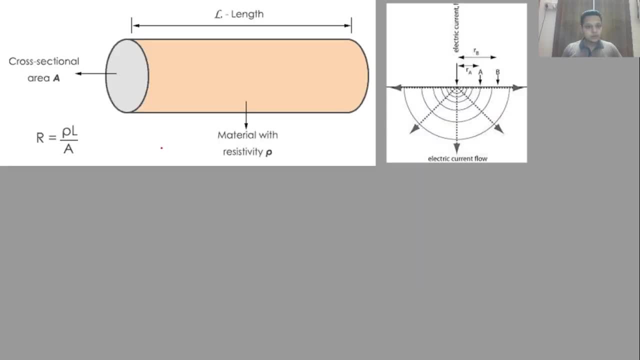 by using this technique. So to understand this, we need to have a very basic idea of the ohms law, which suggests that V is equal to current multiplied by the resistance. Now the reason why? because we are not using the resistance and instead of that we are using 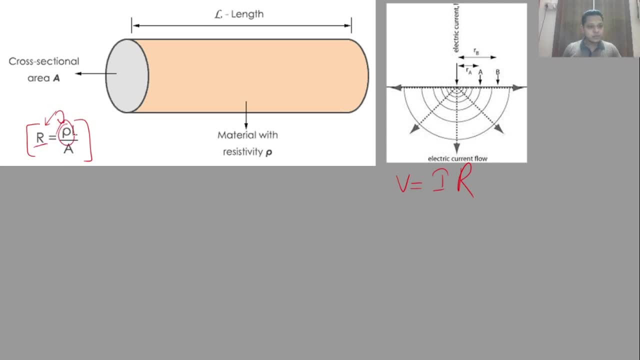 resistivity is that resistance is purely dependent on the dimension of the material you are dealing with, But resistivity is something which you can actually relate to the density, which is an intensive variable. This is only going to change when your material is being changing, is being changed. 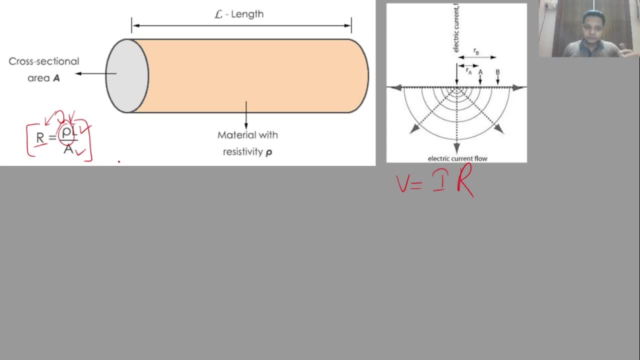 or we can say: the rock is being changed, So the change in resistivity will directly be incorporated into the change of lithology. Now, as I mentioned that we will use the simple ohms law to derive an expression of how we can calculate the voltage of the material, So we will use the simple ohms law to derive. 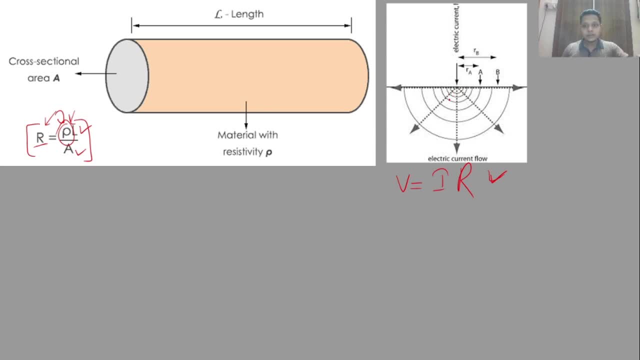 voltage and indirectly the resistivity at any point on the surface of the earth. So let us assume that if we put an electrode, current electrode, over here on the surface, so it will generate these wave fronts of spherical or hemispherical we can say, because on the 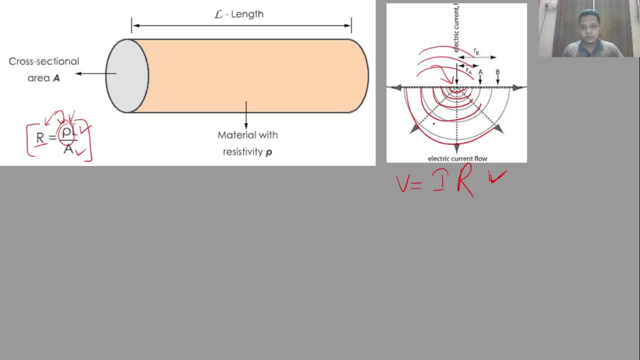 surface of the earth or above that in the air, current won't flow. So this will produce a hemispherical in the 3D wave front which will dissipate like this, radially. Now if I were to calculate the volt, or we can say potential difference at any point, 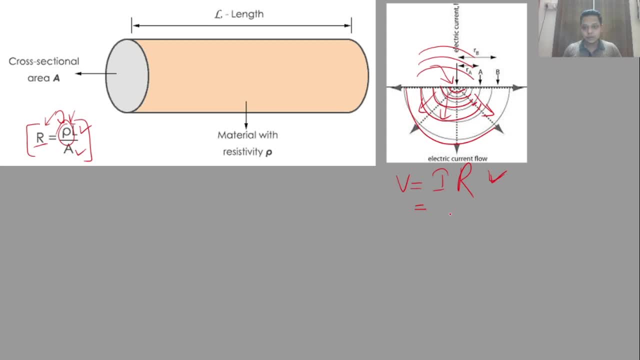 let us say which is r or dr, distance apart, I can write this formula as I, and here also I can write resistivity instead of resistance, as shown by this formula. So I can just simplify this for a time bit and I can write resistivity from here as resistance. 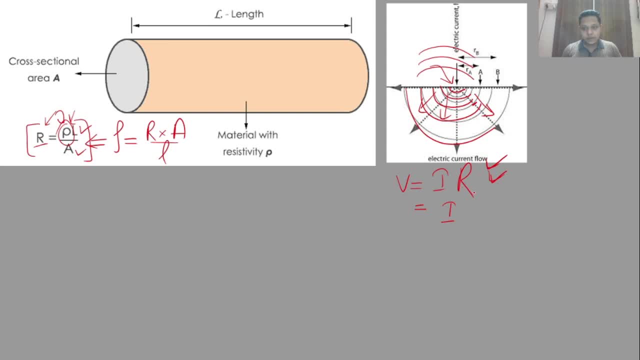 multiplied by area over the length. So I will write resistivity, So I can write resistance as rho into length divided by area. So as this is a hemisphere, I can write the area for that as 2 pi r square instead of 4 pi r square. 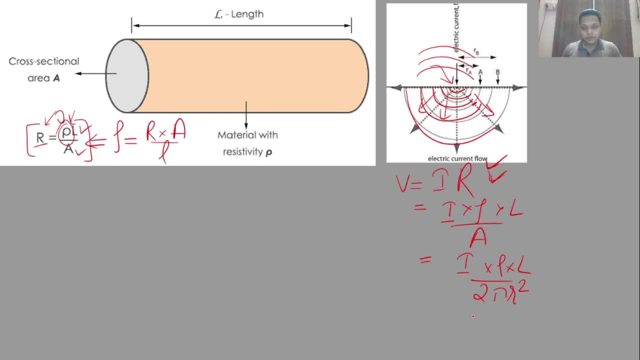 If it would have been the complete sphere, it would have been 4 pi r square. Now, if I am interested to calculate the voltage at, let us say, dr, dr, dr, So I will write this length as dr here, and also the change in the voltage, because, as 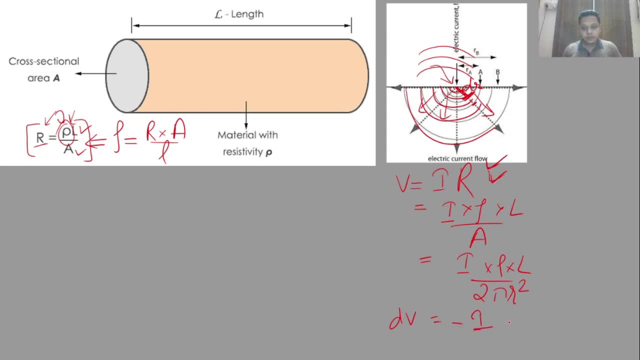 we are moving away, the voltage is decreasing, So I put a minus over here and I can write it as I rho: dr by 2 pi r square. Now, simply, if I were to calculate the voltage over r length, I can integrate both the sides. 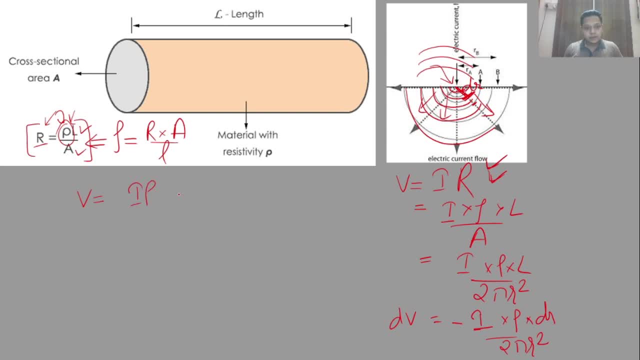 and just simply integrate this dr by 2 pi r square term Right, Okay, So I can put the value of limits as 0 to v and 0 to r to find the voltage in terms of r, so that I can calculate the voltage at any particular distance from the source. 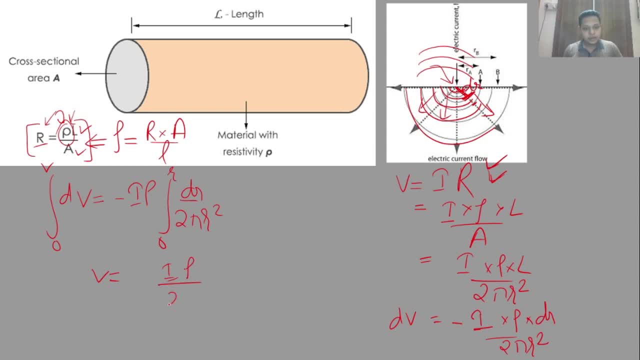 So this will come out to be: I into rho divided by 2 pi r, because the integration of r raised to the power minus 2 will be minus 1 by r and this minus will be accommodated by the minus. Okay, In this sense we already have. 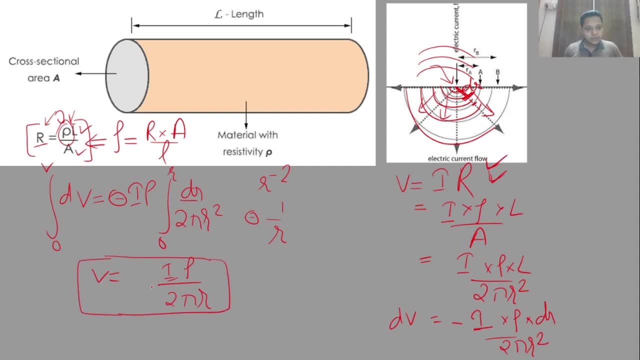 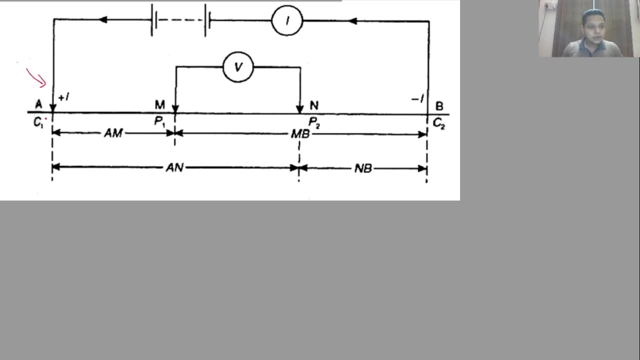 So at last we will have a very simple relation of voltage, or we can say potential, with the inverse of the radius. we want to calculate this potential to Now. I can use this simple relationship to apply the concept for my 4 electrode configuration, in which I am interested in. 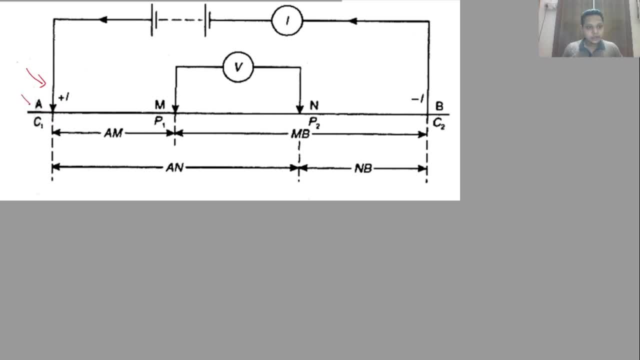 So I have taken two current electrodes and pointed them as a and b in this figure, where my plus i current is equal to 0. is being generated here and minus i over here, and i have two potential electrodes, p1 and p2, marked as m and n here. now the voltage that is going to be generated at m and n will be a. 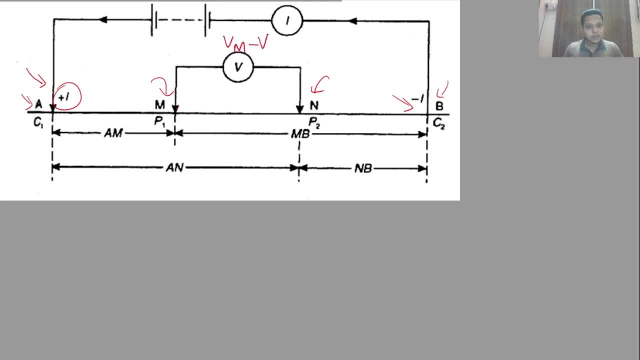 collective voltage, which i can write as vm minus vn, the potential difference, and this vm, this potential at m will be generated by both c1 current and c2 current. similarly, the potential will be generated at n by c1 and c2 current. so i can write the formula for v am, that is, the voltage. 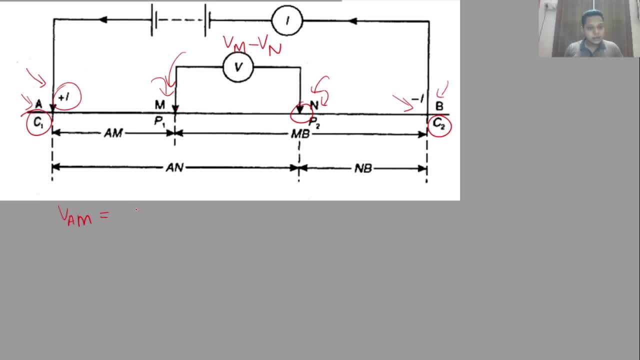 at m due to current electrode at a. simply as i have done, or i have determined in the last slide, as rho into i upon 2 pi r. now here the r will become the am length, because the current source and you are measuring the voltage at point. 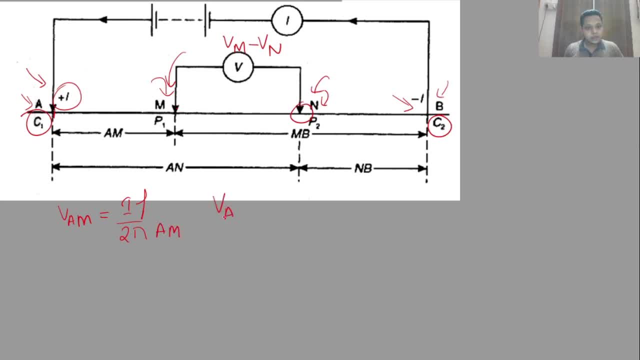 m, so this will become the length. am similarly v b m. you can write as i rho, by 2 pi m b. now i would like to emphasize here that instead of i i will write minus i, because the current which is being generated at b is not plus i, rather it's minus i, because this is a circuit where at one electrode 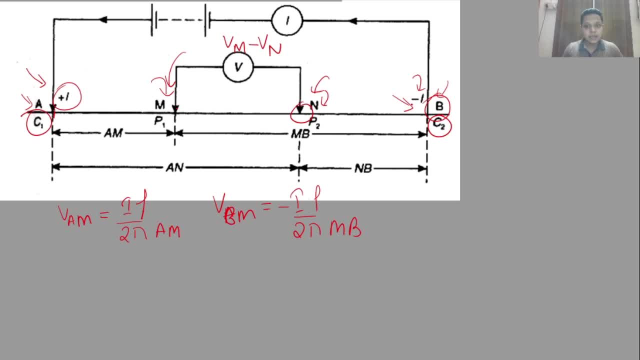 it generates plus current, plus i current, and at another it generates its minus or sinking current, that is, minus i. so collectively at, if i were to write v m, i can write as rho i by 2 pi multiplied by 1 by m minus 1 by v m. so this is the potential which is being generated at point m due to: 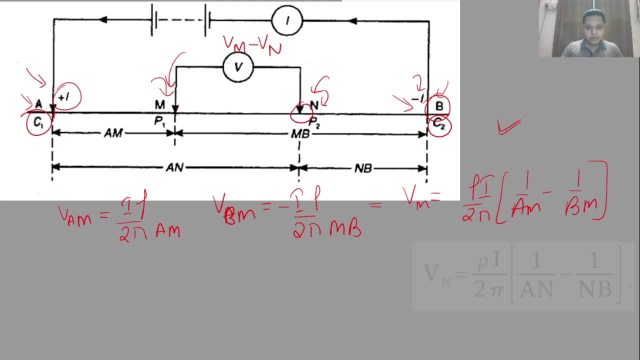 potential or sorry, current electrodes at a and b, and similarly, i can write this formula or this expression for the voltage which is being generated at point n, such as rho i by 2 pi a n minus n b length, in the same manner which we have used for point m. now, as i've mentioned, the calculated voltage or potential. 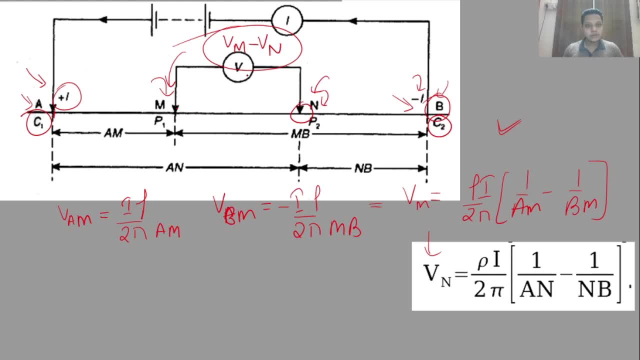 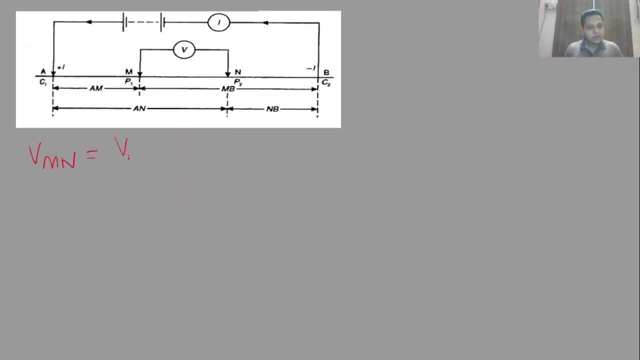 difference at both the points or in this complete circuit will circuit will be v m minus v n. so let's just write that down. it will be nothing but v m minus v n and what we have calculated. i can just write it as it is- rho i by 2 pi, and now I can collectively write it as 1 by a m minus 1 by b m minus 1 by a n. 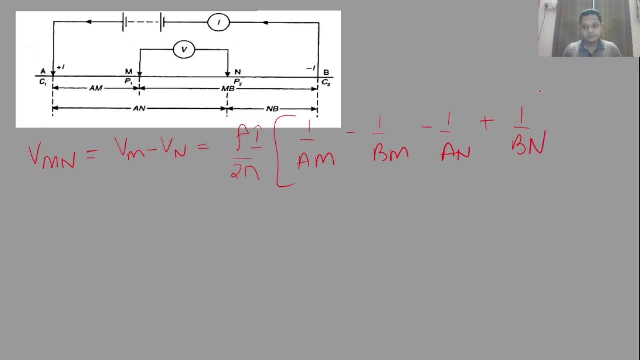 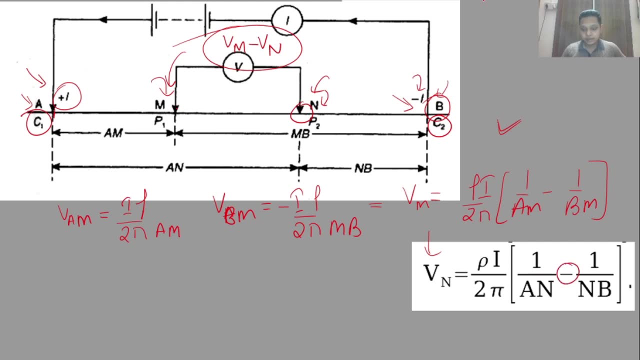 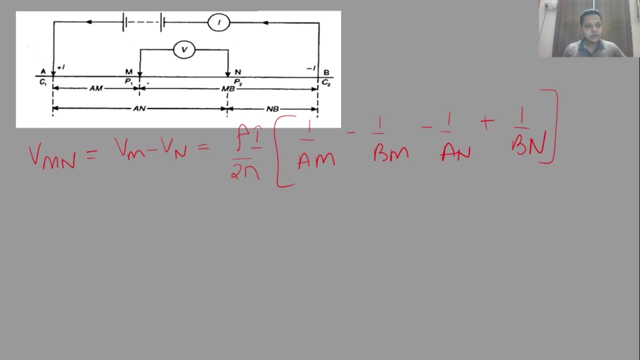 plus 1 by b n. Why this has become plus? Because in the last slide we have seen that it was already a minus and minus minus becomes plus over here. So this is what I am going to get: the potential difference using these two electrodes and using these two potential. 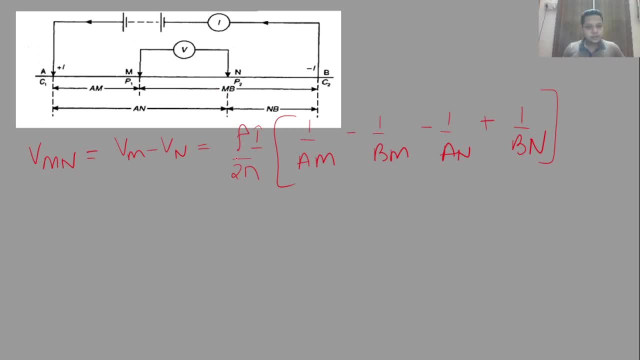 electrodes At last. what I am interested is, what I am interested in is the resistivity. So for that I can write down the formula in the terms of resistivity, in which this whole term, which is simply dependent on the geometry of the electrode configuration, because see if, even for a small, 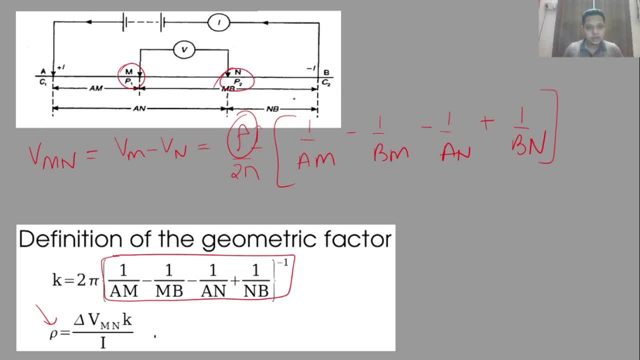 change this- a, m, m, n or a or b- any one of these gets changed, then this whole term is going to change. that is why, collectively, This 2 pi multiplied by this, or the inverse of this, is actually called as the geometric factor, because it is completely dependent on the geometry rest. all the terms are constant: the voltage, the 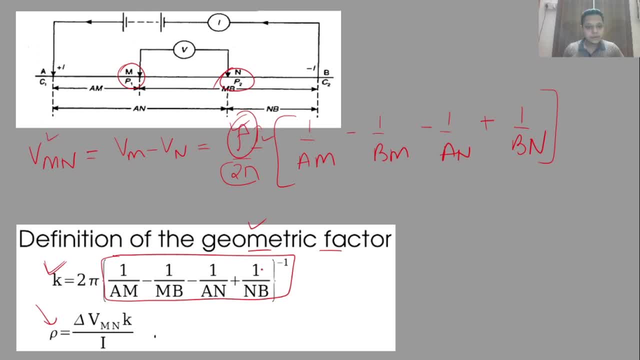 current and the resistivity is going to be constant. So this whole factor- we call it, call it as k or geometric factor, which is only going to be dependent on various geometries you are going to use or you go you are going to encounter. Now, this was a basic idea which you can use. 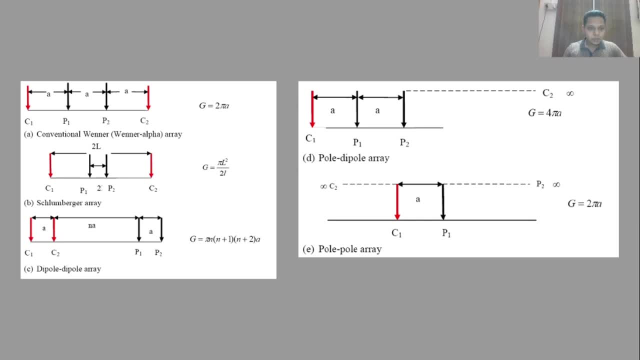 for doing this electrical resistivity survey. now, based on this technique, you can have multiple type of arrays or configurations. most important or most commonly used arrays in industries are the Wenner and Schlumberger array, in which particular the Wenner is, is the one in which 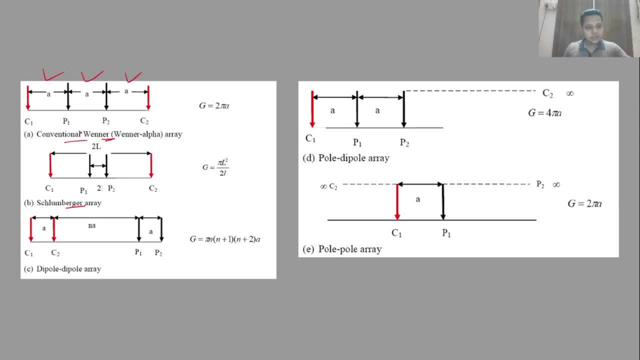 the electrode spacing between current electrodes, the potential electrodes are all same, you can see. So, if you put all these values in the formula we have just derived, you can calculate the geometric factor which is represented here as capital G, which is coming out to be 2, pi, a and. 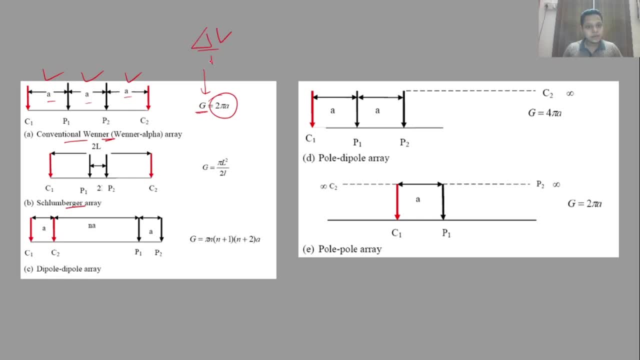 you can just simply write it down as del V by I into the geometric factor which is going to give you the apparent resistivity In the Schlumberger array. the configuration is such that your potential electrodes and current electrodes are quite distant from each other, or or we can say that separation between the potential electrode is quite smaller than. 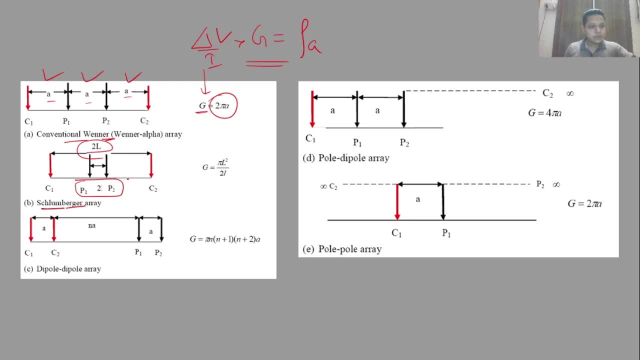 that between the current electrodes. So if you are going to deal with such kind of array or configuration, you will going to get a different formula for calculation of apparent resistivity. Similarly, there are others, such as dipole-dipole, in which you have make two dipoles or you have taken the 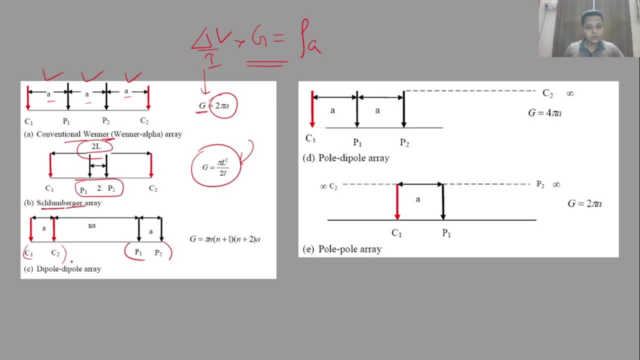 potential electrodes all at one side and current electrode at one side. all these variations you can do for the method or for the requirement. you have the depth of investigation you are going to get. So based on your requirement, you can actually vary these And the most important ones or the most frequently used ones are the conventional Wenner and Schlumberger. 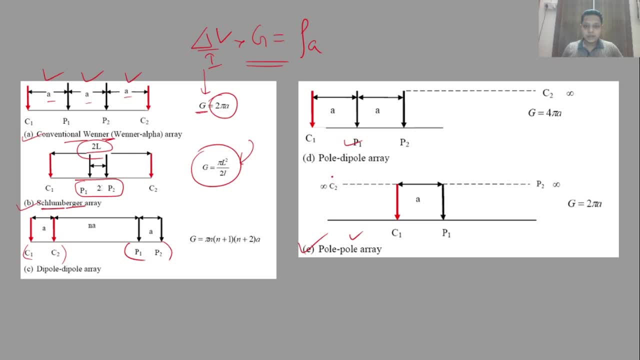 array, But based on the requirement of your survey. you can always change this. you can also, apart from these five, you can actually arrange your electrodes in your own way, based on your requirements. Now, this was the calculation part, or the behind story. what? what actually happens, but what? 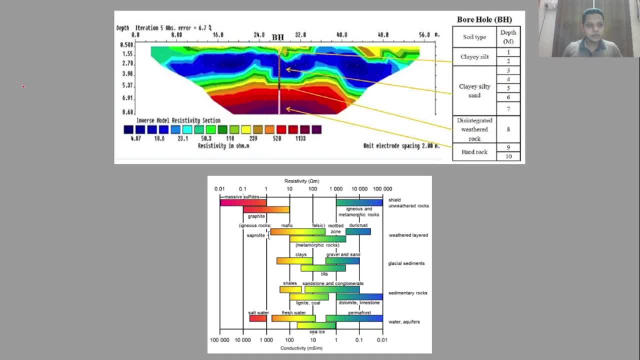 we do after all, or doing all these is the interpretation Part. this is quite important part because you can do the survey, but if you are not good at interpreting the data then it is a waste. So after doing all these survey, you are going. 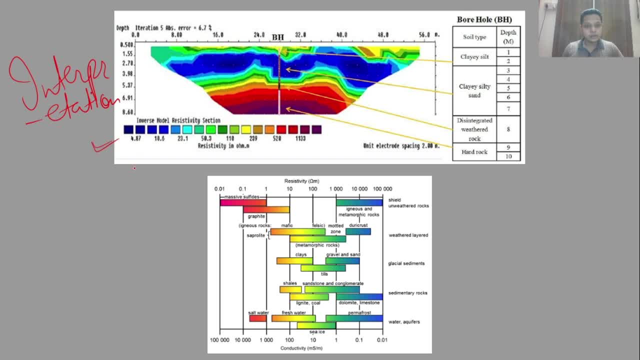 to generate these sensitivity curves, or we call call these as ERT curves- electrical resistivity tomographic curves in which you are going to plot the resistivity data in this color chart, which is mentioning the resistivity in ohm meter scale, where the color of the 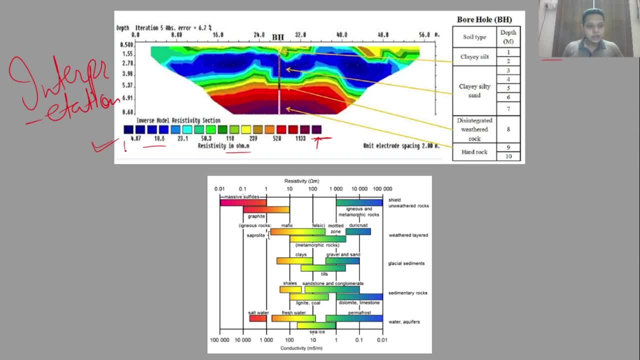 purple is going to give you a very high resistivity value, and the blue, on the other hand, is giving you the smaller values of resistivity. based on this, if you dig a borehole and you encounter such type of resistivity variation, the possible interpretation which you are going to make out of this can be so and so. so this will going to give you a very brief 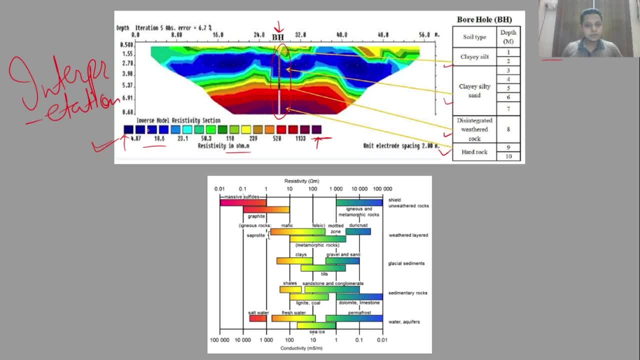 idea, or very good idea, about the lithology that is present and you can see the depth it has. it had encountered is about 9 meters, which is quite good for the exploration of groundwater, and it is being extensively used because we know wherever you will find water you will going to get the 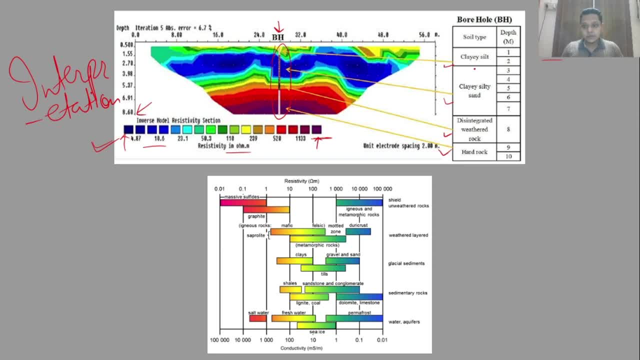 low resistivity. so hence you have these color color chart with you and you can also use different type of charts to mention the different resistivity values. also, you can see that the resistivity variation is quite large. i mean from very low value for of point zero, zero, one ohm meter, to about hundreds of thousands ohm meter, you can have the resistivity. 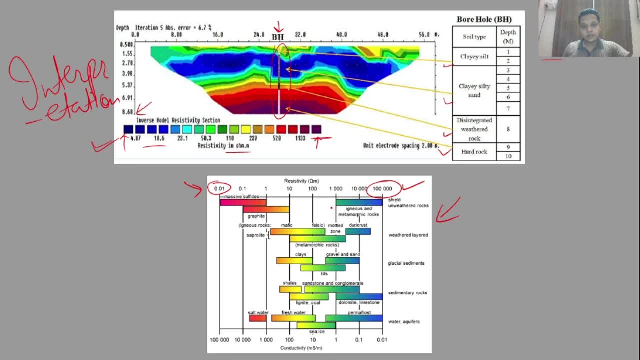 based on the configuration of your or mineralogy of your rock. so resistivity is one physical parameter which is having a wide range of variation. so once you get the resistivity values or the variation in in the subsurface, you can very well correlate this chart with your. 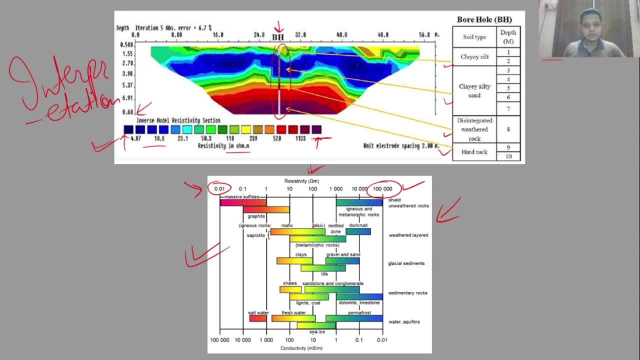 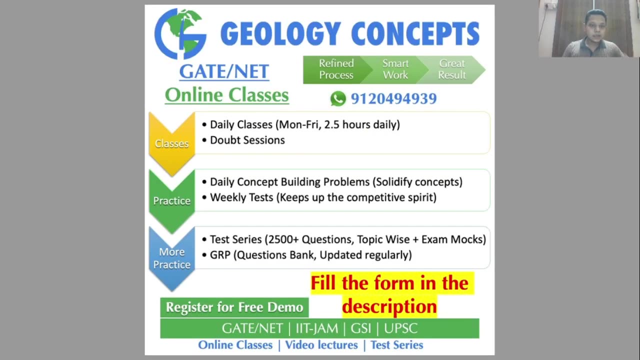 variation and you can have an very good idea about the subsurface lithology. so this is a very brief or summary of how does this type of method is being used in the exploration techniques. so i hope you like the video and also in the last i would like to mention that we have started our 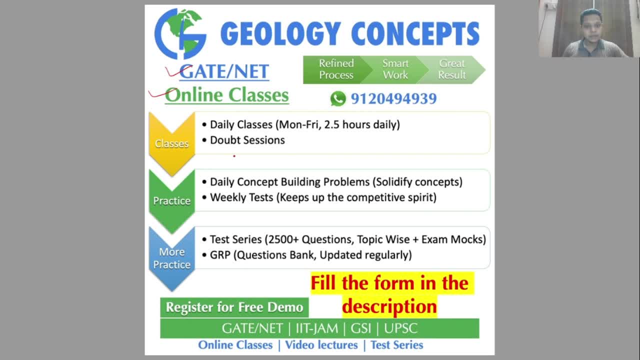 gate and net online classes, which are being conducted daily, monday to friday, and for that you can also join the demo classes that are free of cost. register for those demo classes, fill the form in the description given down below, and also, if you like the video, please share it with your. 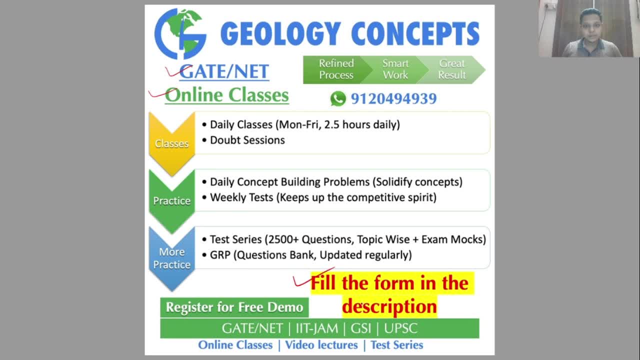 friends, subscribe to our channel and we will see you in the next video. bye, bye, channel, and stay tuned to geology concepts. thank you so much. have a nice day. 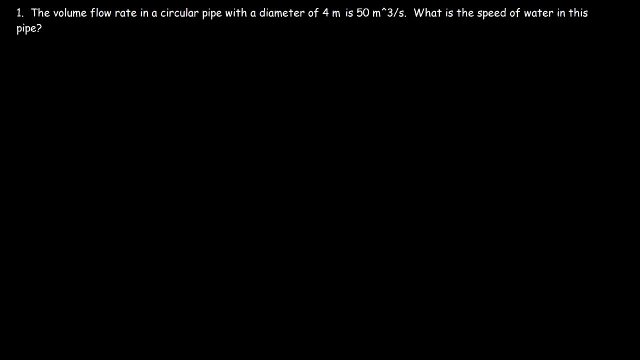 Let's start with this question. The volume flow rate in a circular pipe with a diameter of four meters is 50 cubic meters per second. What is the speed of water in this pipe? So let's draw a picture, And so here's the pipe. If the diameter is four, that means the radius has to be two meters. 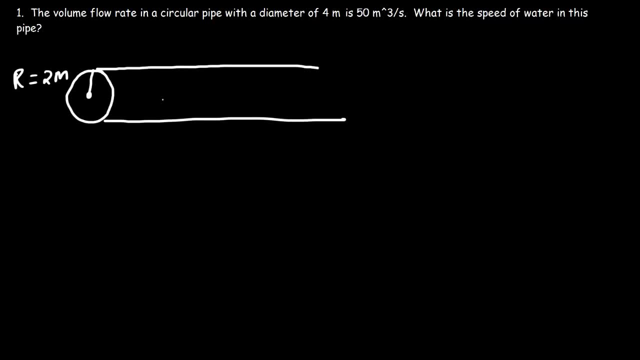 And the volume flow rate, which is the change in volume divided by the change in time, that's 50 cubic meters per second. So how can we use the volume flow rate to calculate the flow speed in the pipe? Volume is area times height. In this case, the height could be just the horizontal.